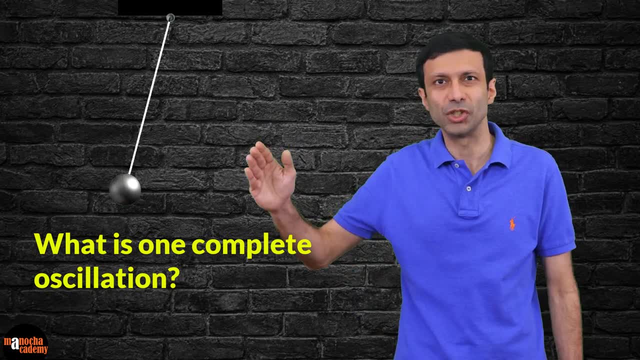 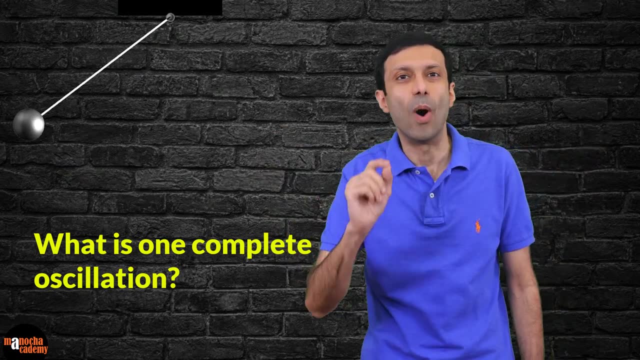 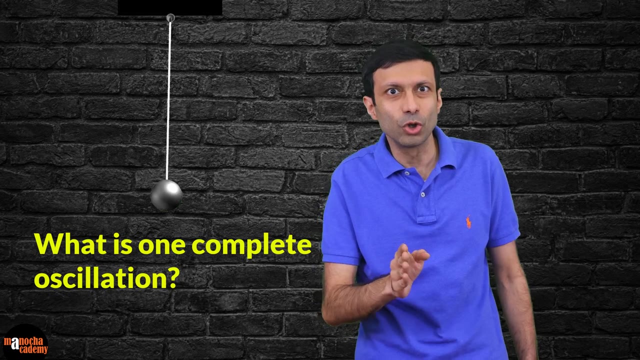 If you start the pendulum from one extreme position, so when it swings and comes back to the same extreme position, it is called one complete oscillation. Or if you start the pendulum from the center position, then the pendulum goes to one extreme position and then it swings back and 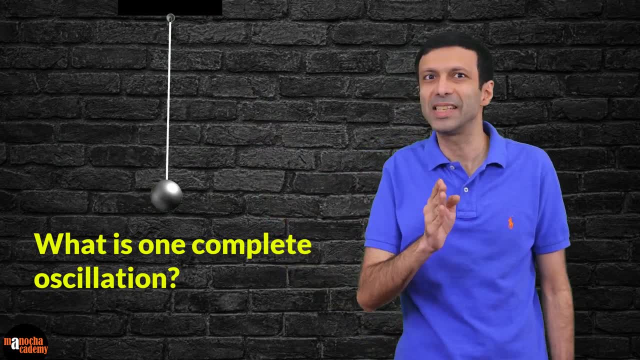 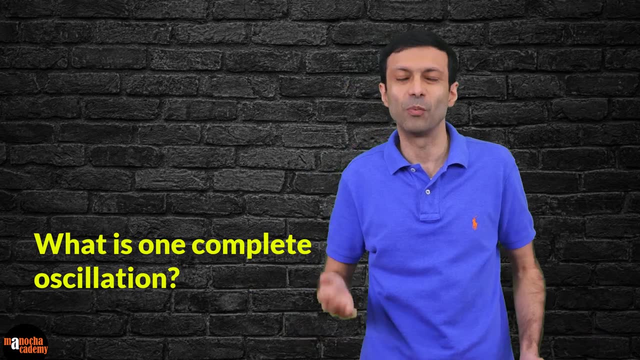 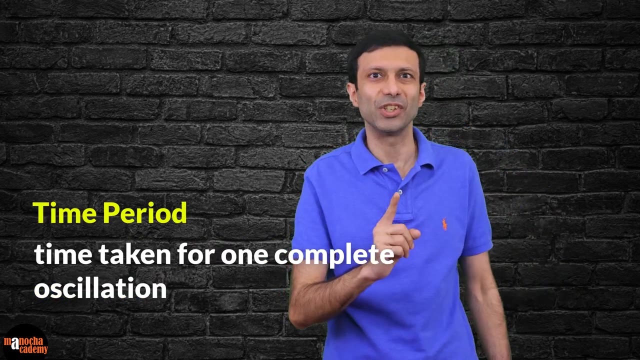 goes to the other extreme, and now it must come back to the center again. That is again one complete oscillation. So whichever way you measure it, from, whichever position, that's a complete oscillation. Now, the time taken for one complete oscillation is called the time period. Let's say: 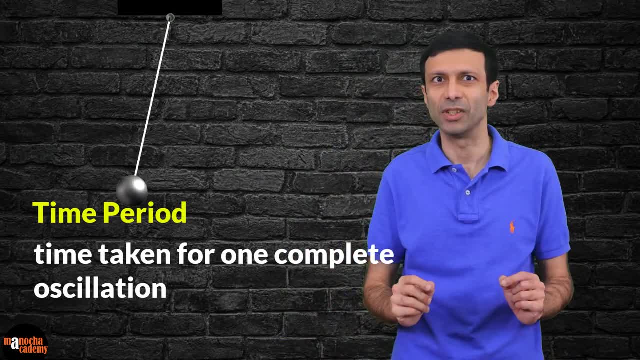 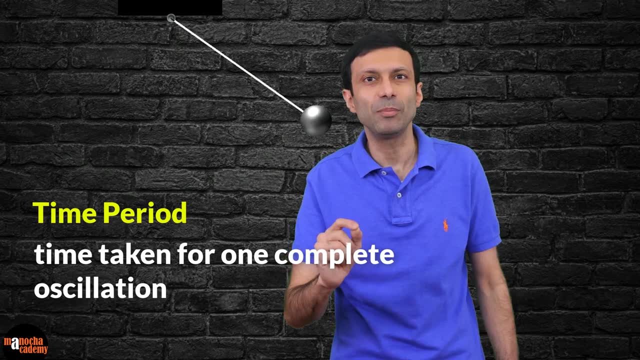 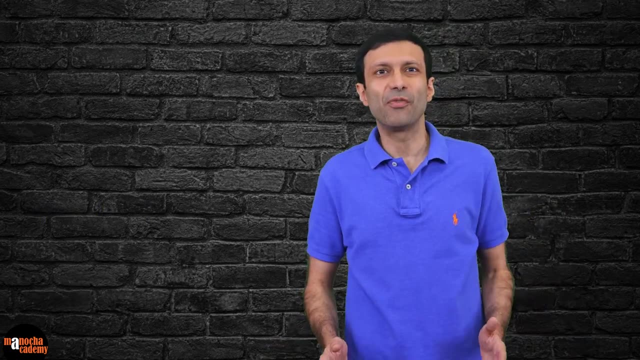 the pendulum took two seconds to complete the oscillation, Then the time period is going to be two seconds. Remember, the time period is the time taken for one complete oscillation of the pendulum. O is called the time period of the pendulum, Then frequency is defined as the number of oscillations. 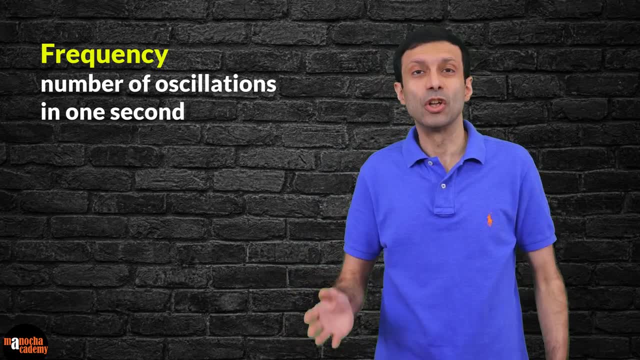 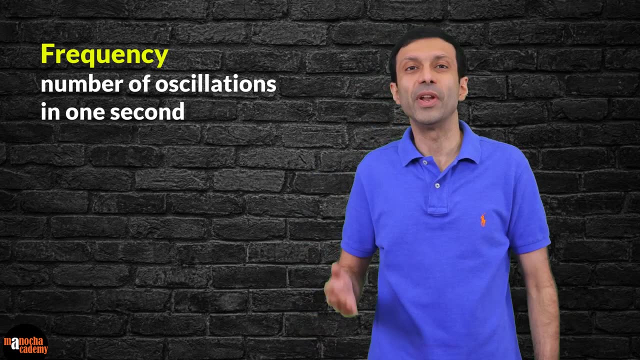 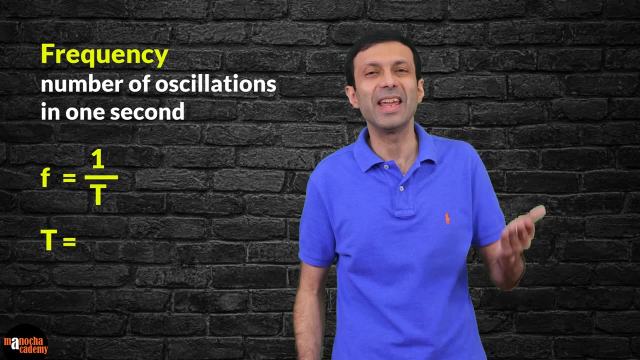 in one second. So frequency is the reciprocal of the time period. So what is the formula going to be? F is 1 by T. Or we can write time period: T is 1 by F. the frequency Now what is frequency for pendulum? 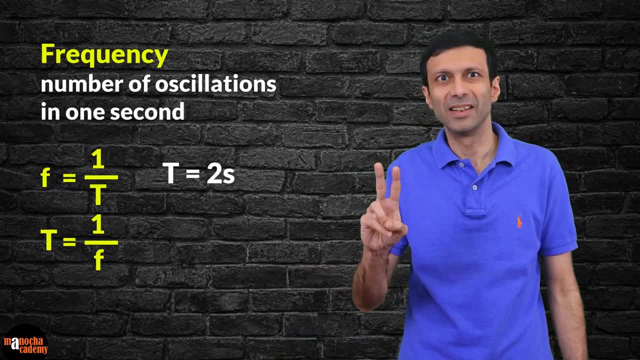 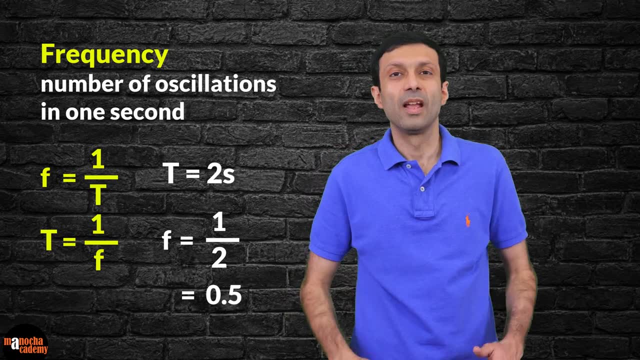 whether time period, Simple distinction, or time period over frequency of frequency. Sun byτέs losae was 2 seconds. That's right. if you take the reciprocal, the answer is going to be half or 0.5, because it is completing half an oscillation in one second. The 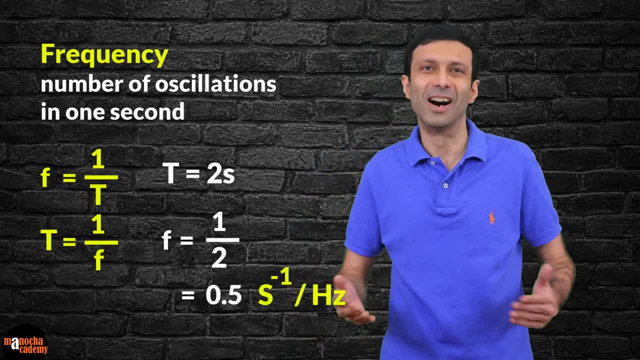 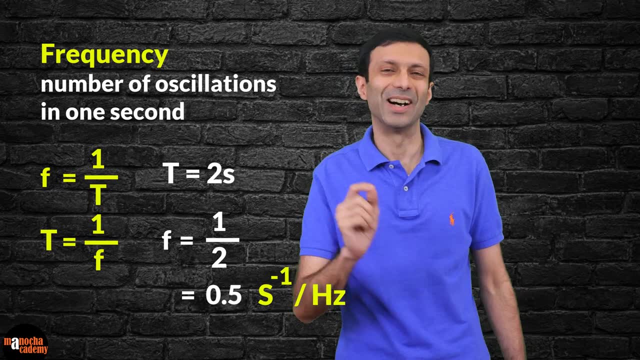 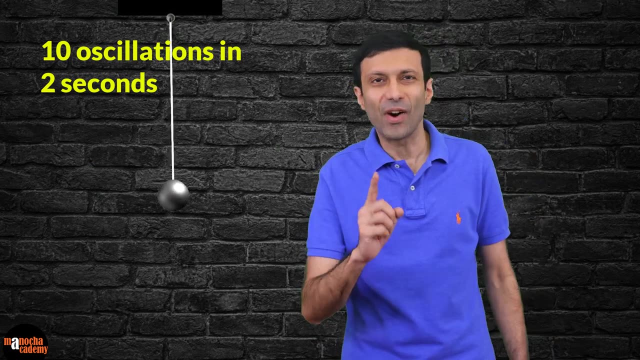 unit of frequency is second inverse or Hertz. So the frequency of our pendulum is written as half Hertz or 0.5 Hertz. Let's say a pendulum completes 10 oscillations in 2 seconds. Can you find its time period and frequency? 10? 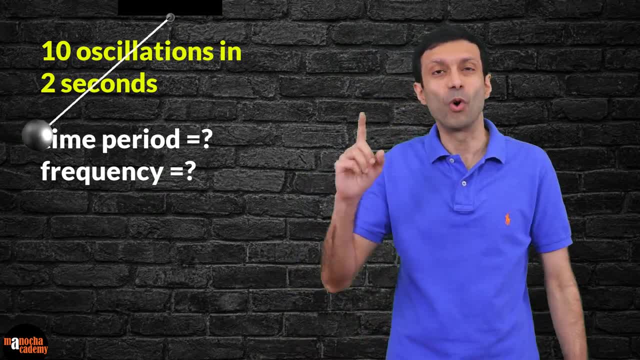 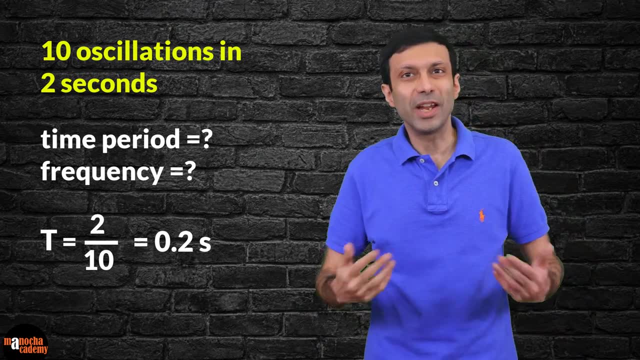 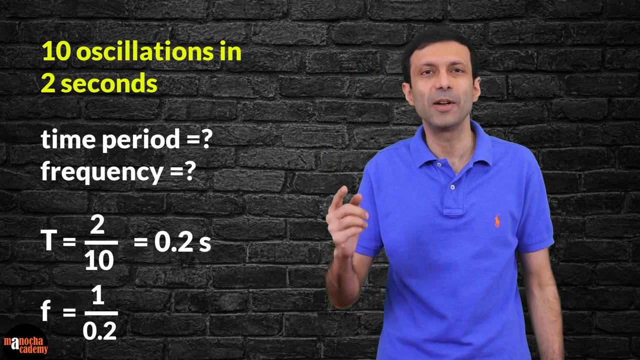 oscillations takes 2 seconds. So the time for one oscillation is 2 divided by 10, which is 0.2 seconds. Frequency, as we learnt, is the reciprocal of the time period. So the frequency is going to be 1 divided by 0.2, which, if you.